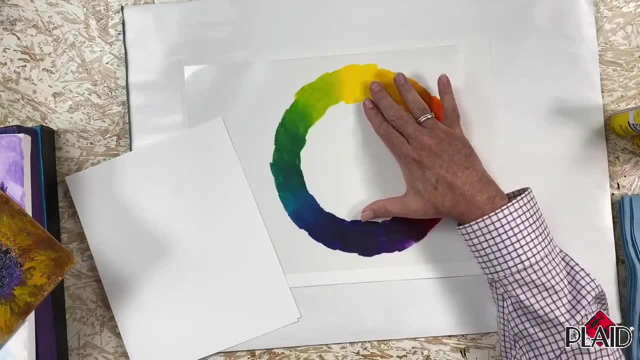 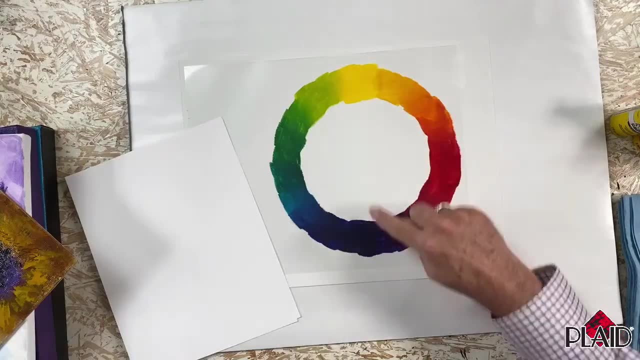 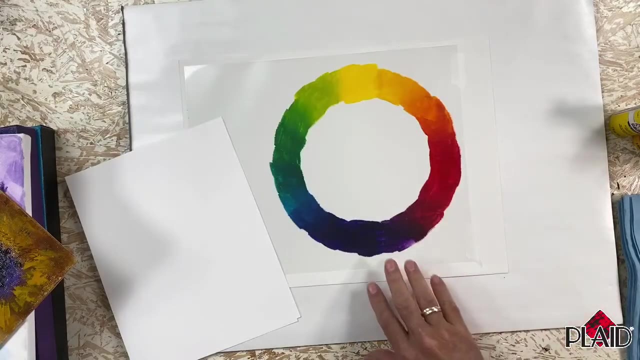 in not only color but also value. So purple or violet is generally much, much darker than yellow, which would have a light value. So this is intense contrast, both in terms of hue and value. All right, so you could also do. blue and orange is a great complementary color scheme. 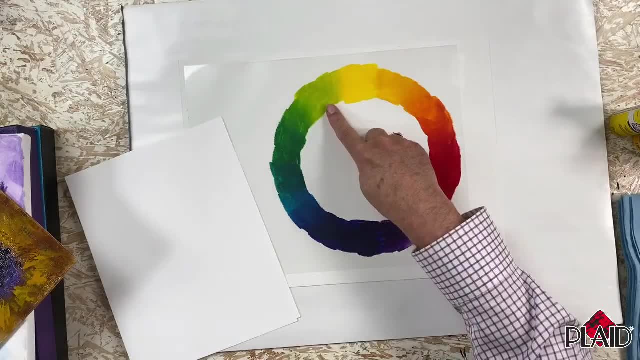 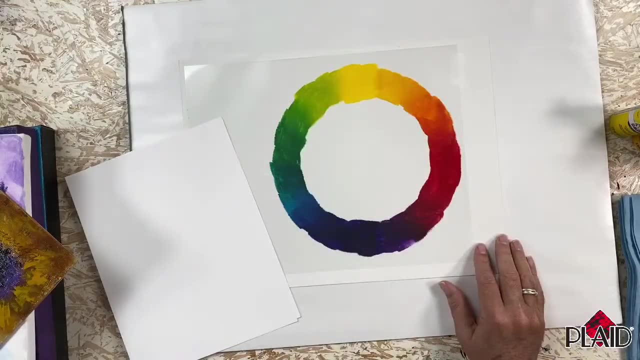 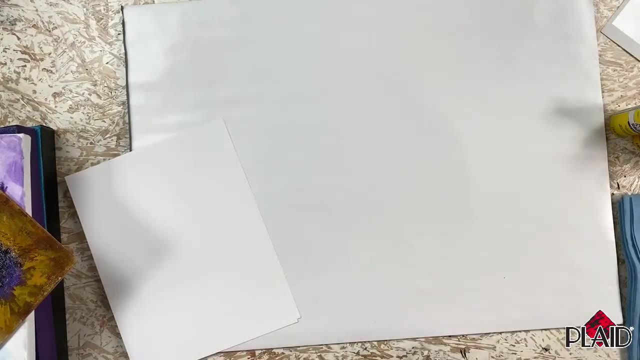 Green and red is a great complementary color scheme. You could also do yellow-green and red-violet. Any color that lies opposite the color wheel will give you a complementary color scheme, But today it's all about yellow and purple. So I want to give you a little thought to keep in mind as we look at a couple of examples. Only one color is a complementary color scheme. 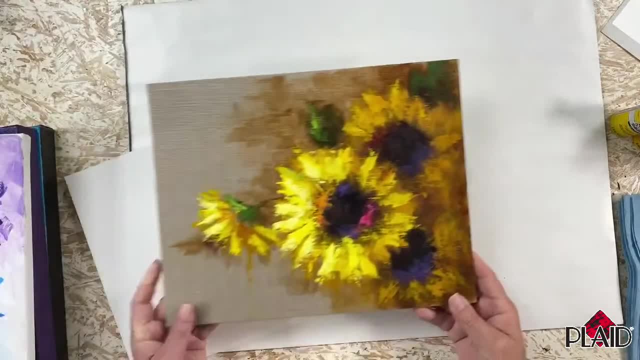 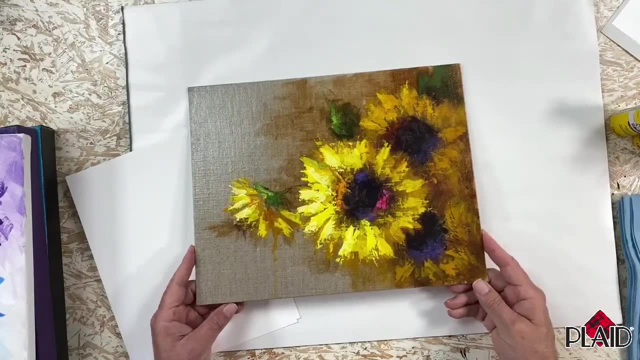 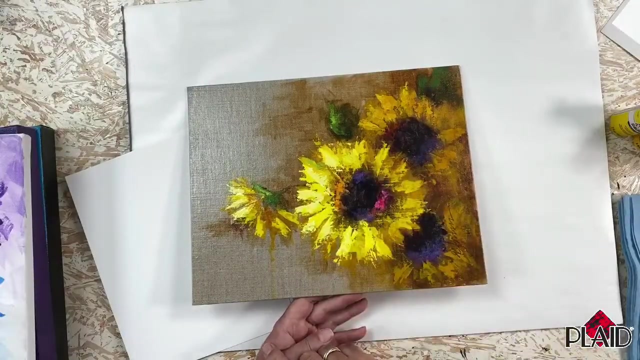 Yellow can be the star of the show, All right. so here is an example of a painting of sunflowers, And you might look at this and just think it's a sunflower painting, but it is actually a complementary color scheme because we have yellow and we have lots of violet in our painting. 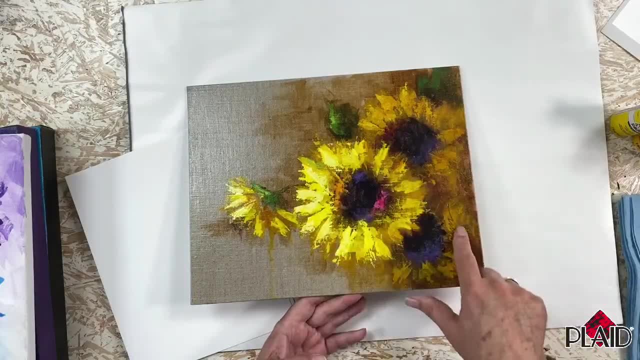 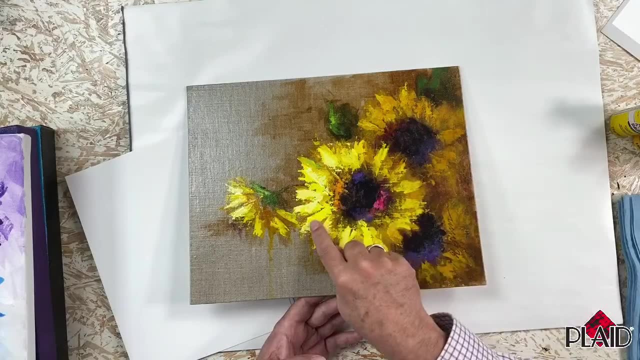 We've got lots of different values of yellow, lots of different intensities. So we've got dull yellow and we've got bright yellow, we've got dark yellow and we've got light yellow. So lots of stuff going on with our yellow, but the complement that gives it a nice foil. 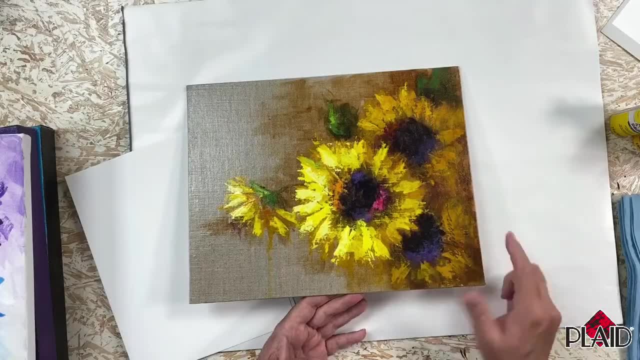 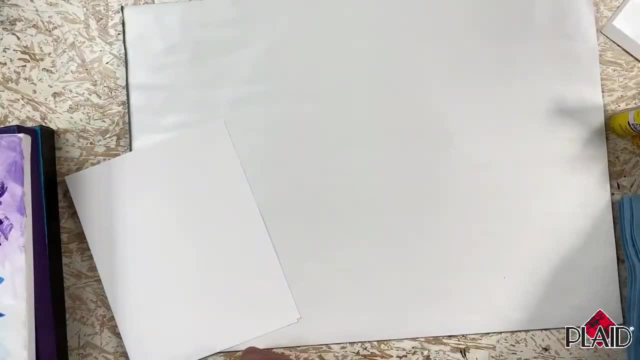 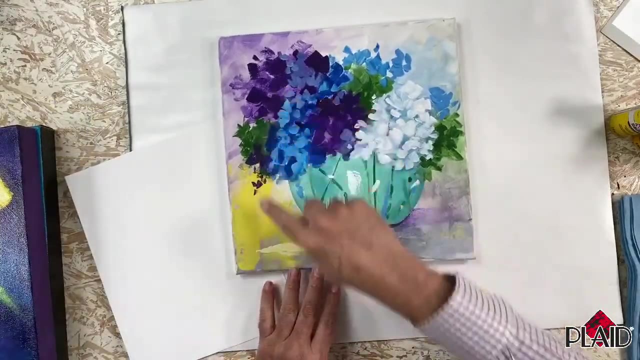 is our addition of violet to this painting, So yellow is the star of the show here. All right, so we're going to set this aside and we will bring in another example. So if you look at this particular painting, it's very easy to see our yellow and purple. 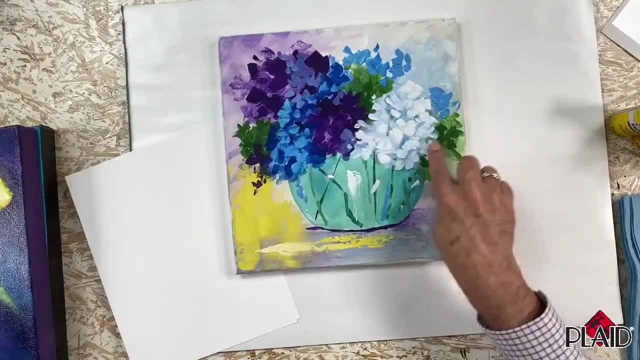 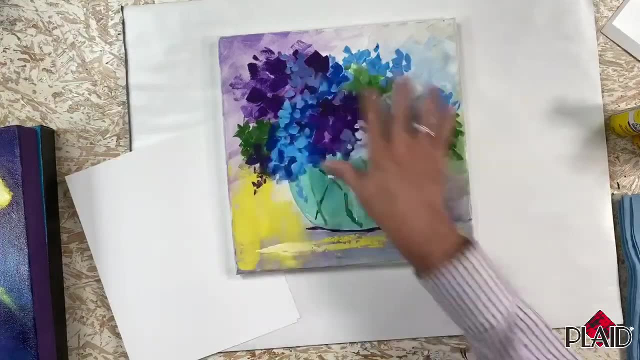 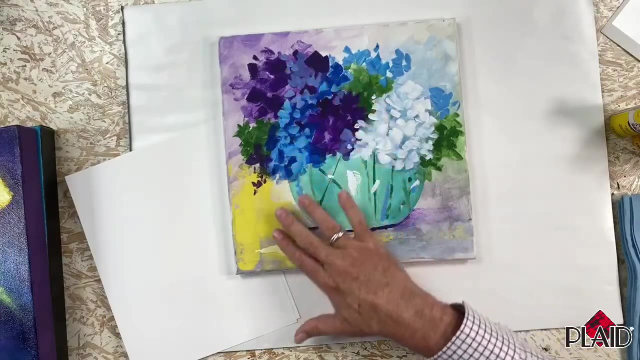 complementary color scheme going on here, But we also have some supporting color schemes. We have a supporting cast of characters in here, with some greens and some blues to make it an overall composition. But really the big star here is our complementary color scheme, with the yellow probably being the brighter star of this show as well, even though there 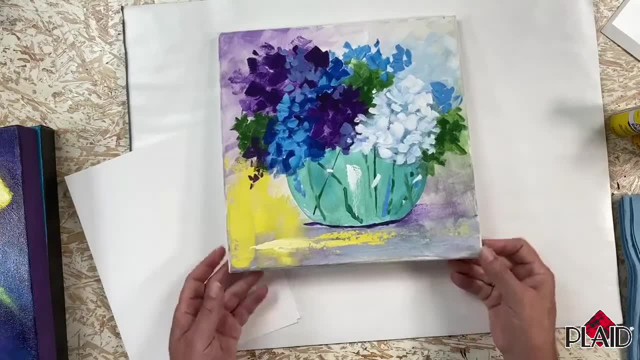 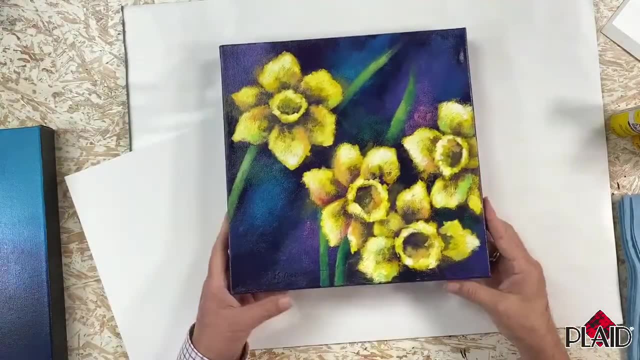 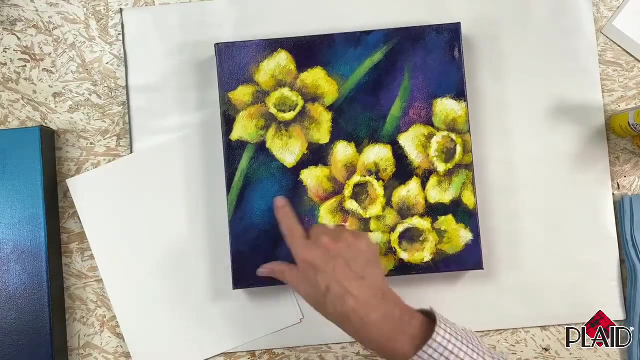 is quite a bit of purple there. All right, so just pointing some things out as we look at some examples before we start in with our little mixing. So here is another example of that painting that we did. that's a beautiful complementary color scheme and we have lots. 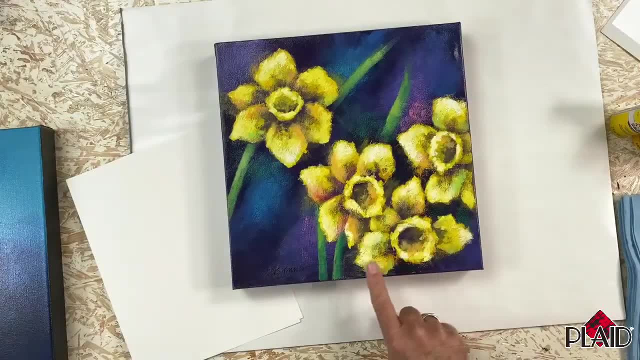 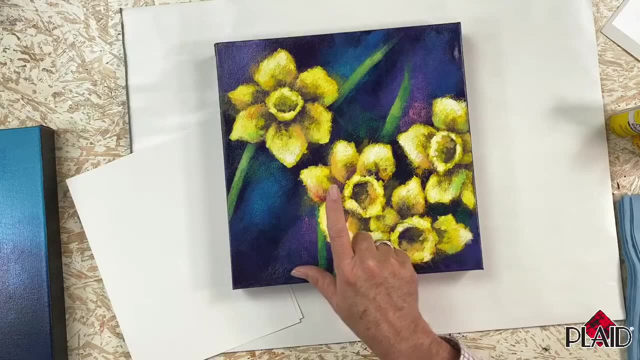 of purple in the background. Once again, the yellow is the star of the show and we have more things going on with our yellow, lots of different values of yellow going on, and we've got some orange accents in our yellow flowers and we've got some blue accents in. 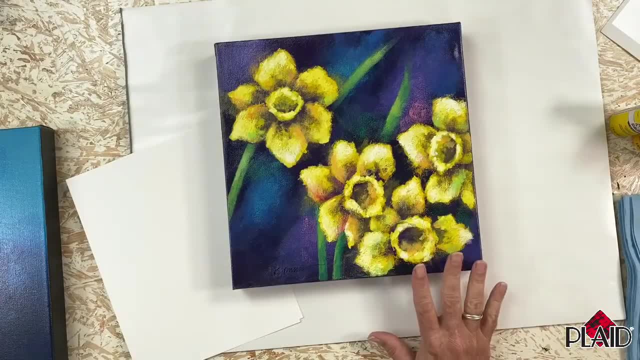 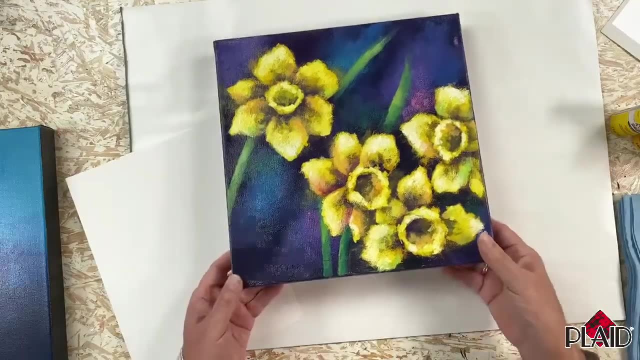 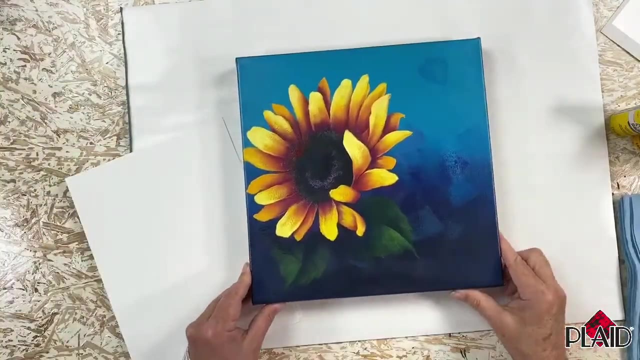 our purple background. So good example of making a yellow and purple color scheme not be boring. All right, because you never want a boring painting. You always want your viewer to be entertained. Here is another yellow and violet. Let's turn this right way for you all to see. 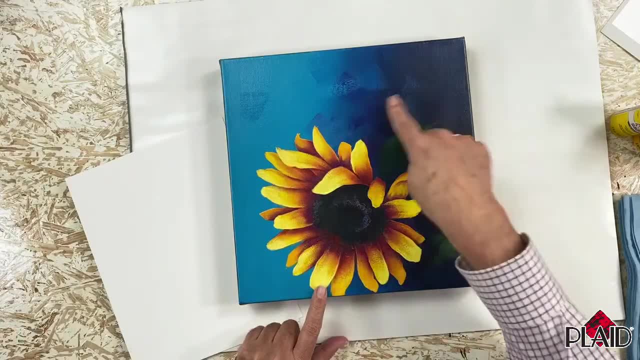 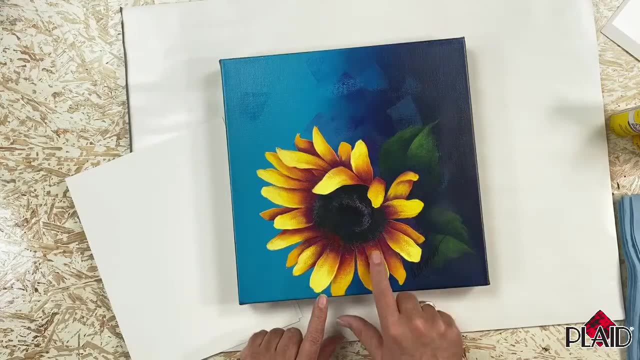 this. So we've got lots of yellow going on here and there is blue and purple in the background. So again we've got bright yellow, which is the easiest way to make yellow the star of the show, and the purple recedes into the background. But you could have a 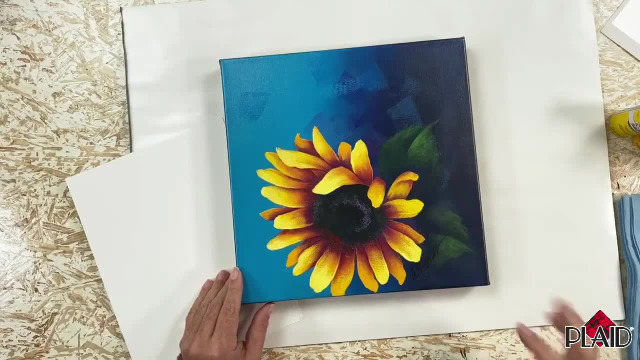 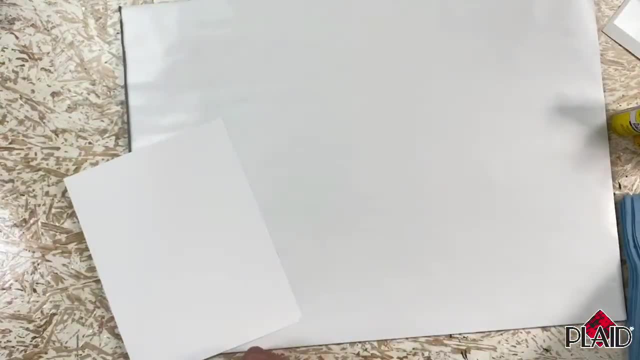 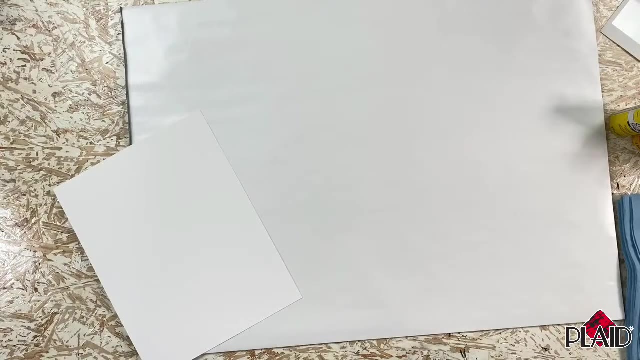 painting where the purple is the big star of the show and the yellow is secondary to that. So we're going to talk a little bit about that. but I want to give you another little expression or a little saying to help you with this, and that is: don't let your. 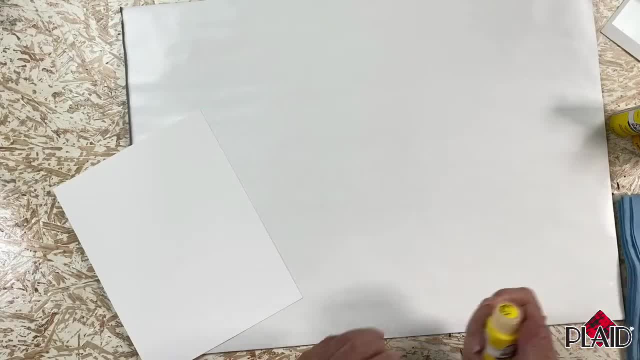 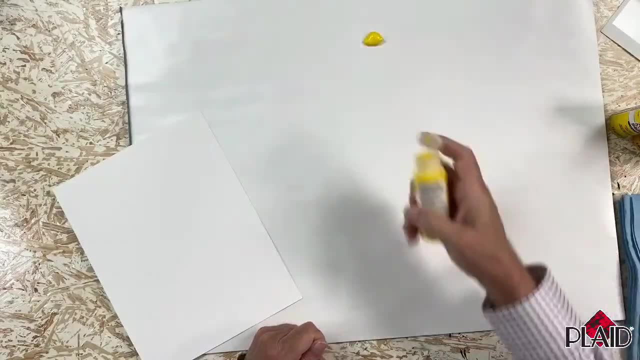 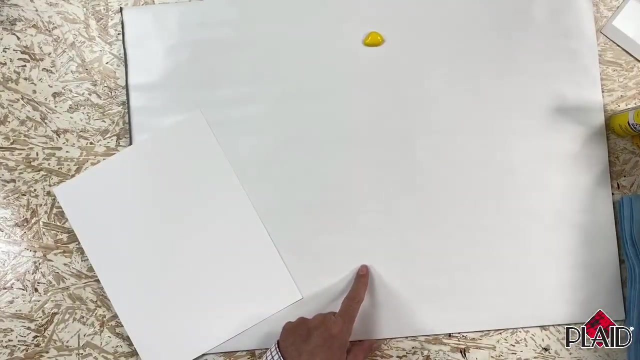 guidelines be your girdle. You can take all of these rules and you can bend them and do what you need to do to make a really attractive painting. But only one point of reference, only one color can be the star of the show, So I've put out a yellow here on my palette. 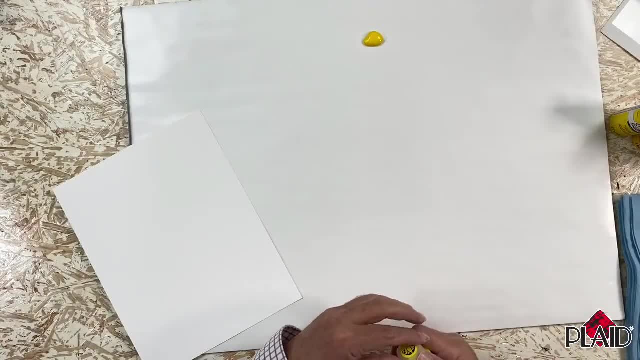 and it doesn't really matter what yellow you have, because these rules will translate to lots of different colors. But I am going to just squirt out a number of different yellow colors here so that you can see that it doesn't take much to have a big variety of yellows. 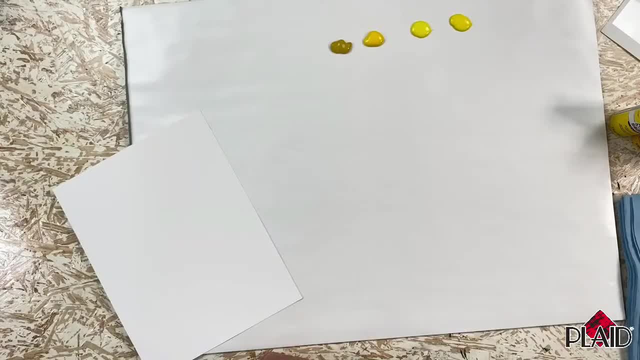 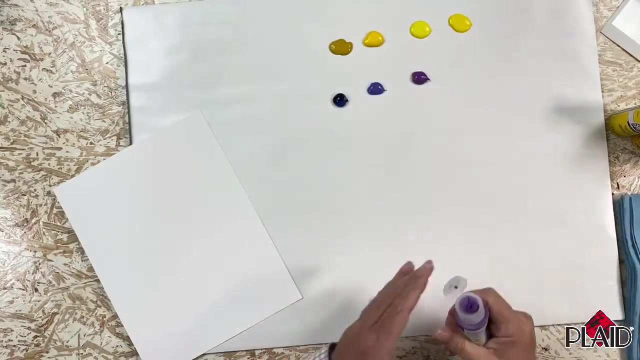 All of these are great yellow colors, and let's put out some purples too, so that we can just do a nice contrast of colors here. Lots of colors to work with, and we're going to do some mixing And I'm going to paint some swatches out for you to see things, But this color here is. 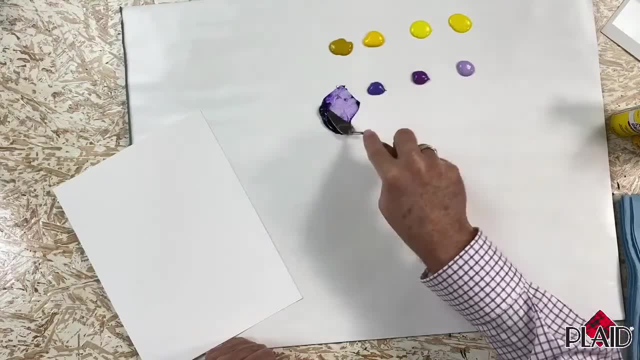 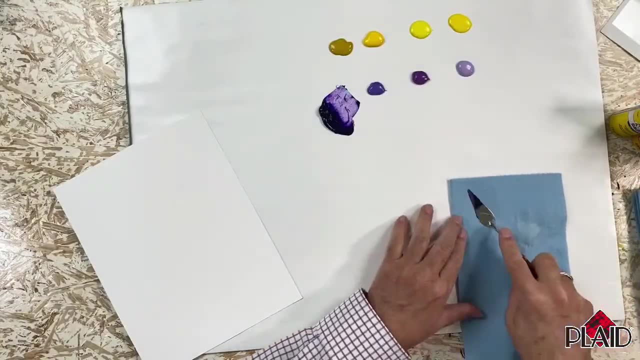 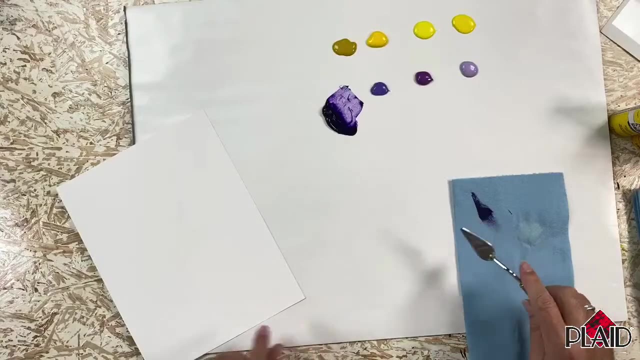 dioxazine purple and it is super, super dark. This is what you think of when you think of a purple color on the color wheel. It is dark, it is intense and it is bold and will take over unless you contrast it. Let's start here on our little sample sheet, just to show you. 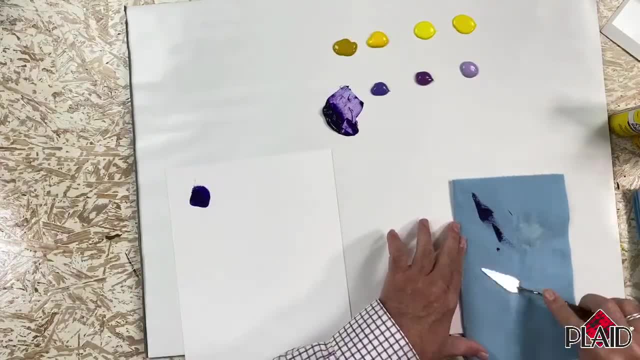 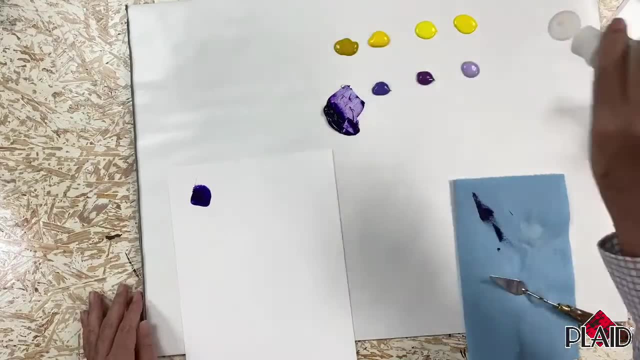 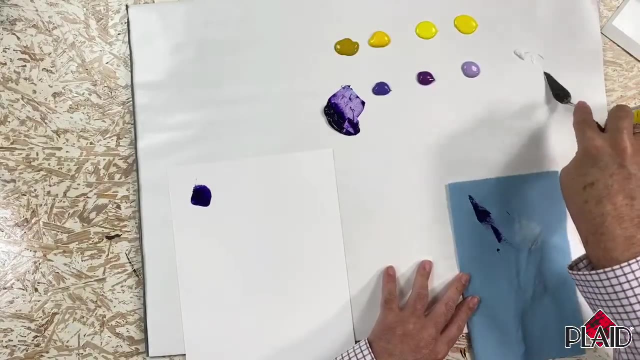 We've got a nice purple there. I am going to put out a little bit of white on my palette so that you can see how we can reveal this color. So I'm going to take just a tiny bit of white here and just lighten the edge of this so that you can see. 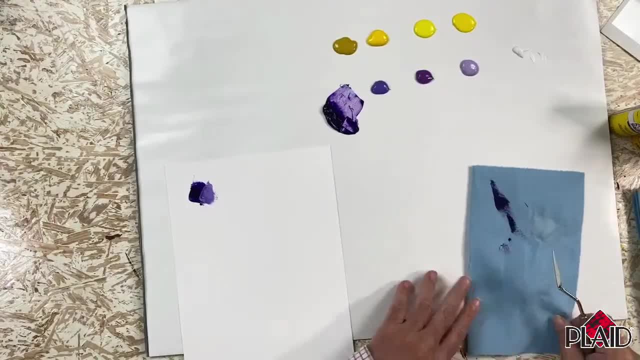 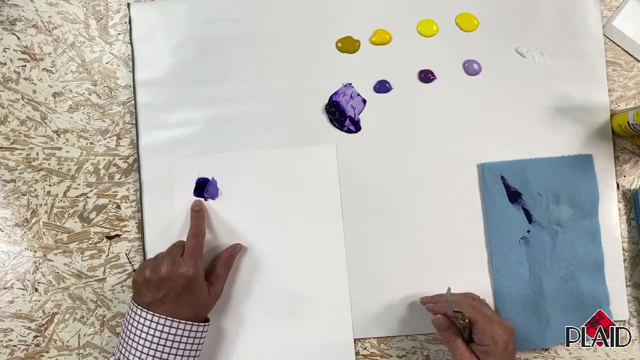 what that color really is. So any time you're doing like a color chart or you know painting something out for reference material, if your color looks black when you're just looking at it, go ahead and add a little bit of white so that you can reveal the 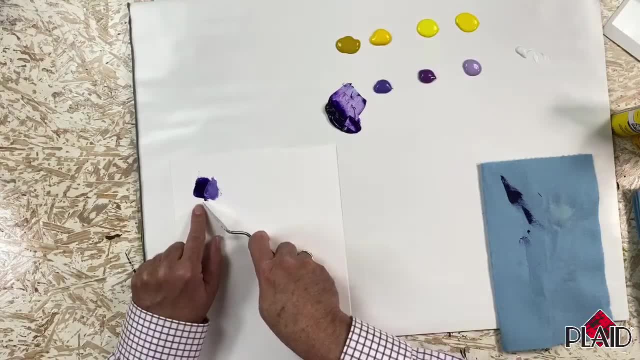 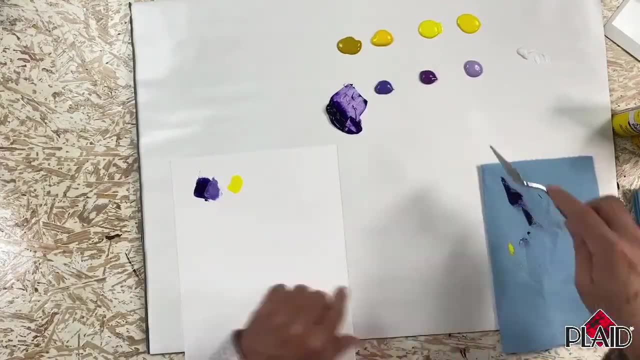 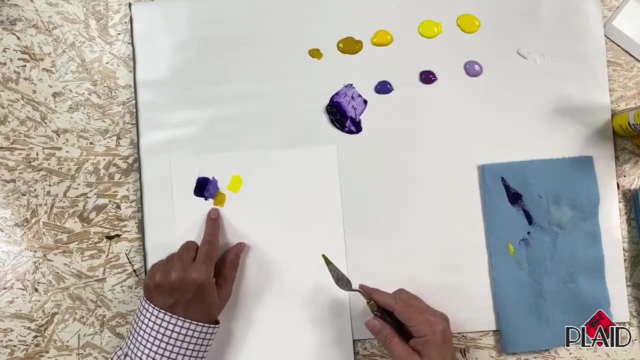 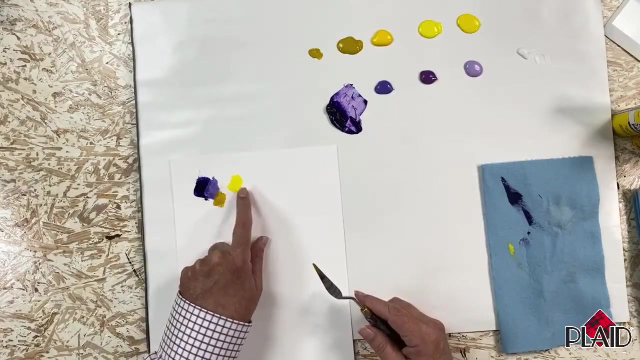 color to know what that is. but to coordinate with this, we could use an extremely bright yellow. that's one option. or we could come back with a more toned down yellow and you can see how much easier this yellow rests next to the purple than this one does. this is creating high drama, high contrast and 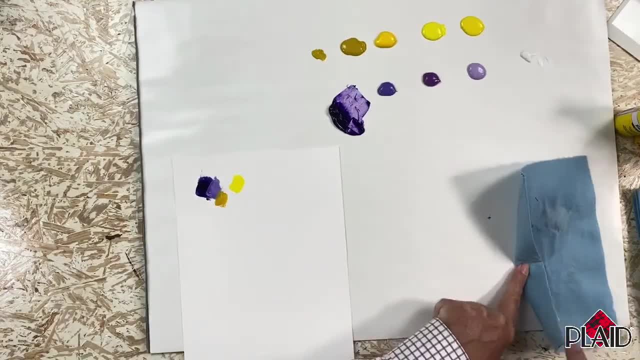 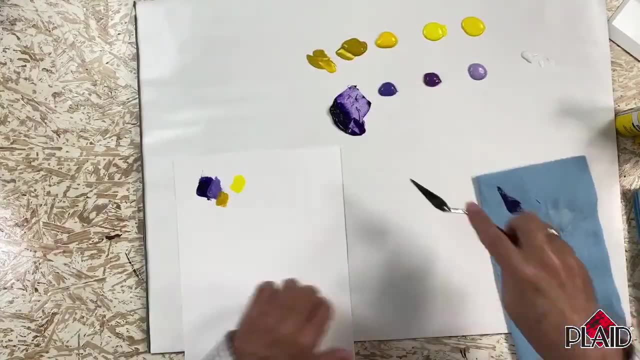 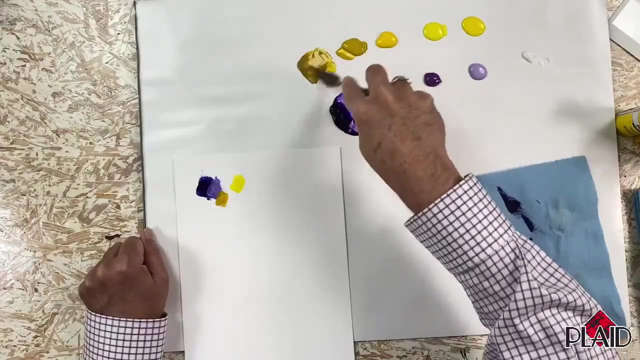 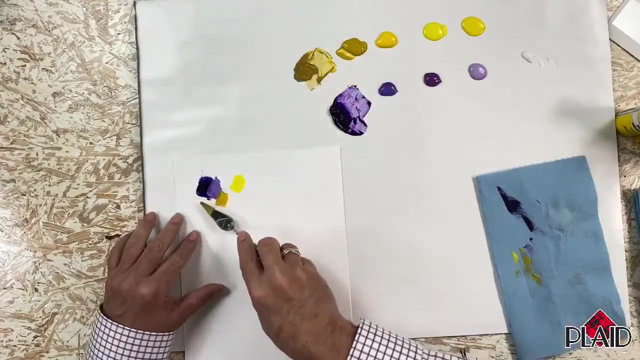 this is more subtle and easier on the eye. so if you're using a color that is already toned down, we can take that a little bit further and actually add some purple to that yellow and we can create a nice golden color here which will sit very, very nicely next to that purple. And you can 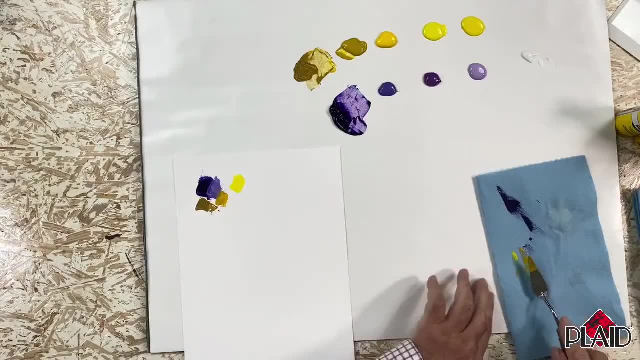 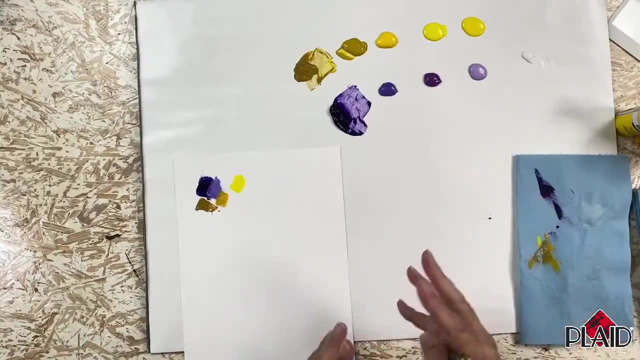 make the purple the star and this kind of yellow kind of recede into the background. So if you were painting a composition of purple grapes and lemons, you can decide whether your bright purple grapes are going to be the star of the show and your lemons are. 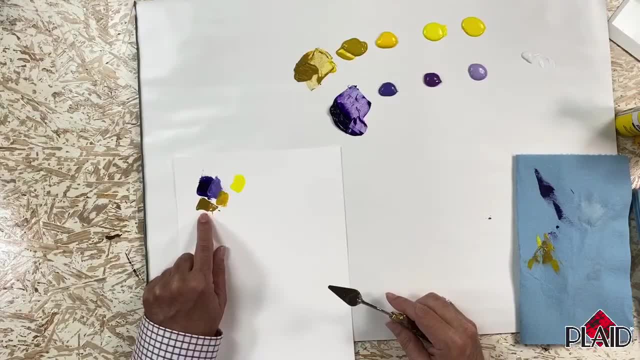 going to be toned and shaded with some of the purple, and you can even add some rusty accents in there so the fruit doesn't look rotted. but you can make the grapes the star that way. Or if you want your lemons to be the star, then you'd have dark purple grapes. 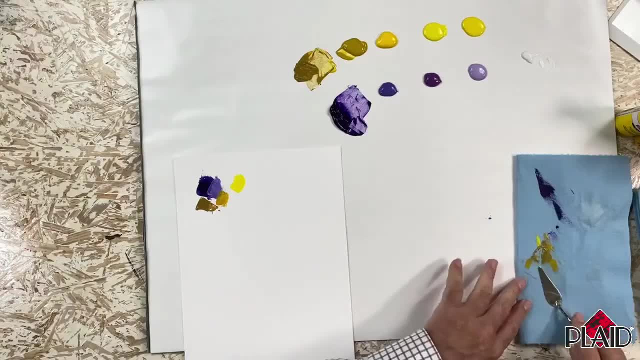 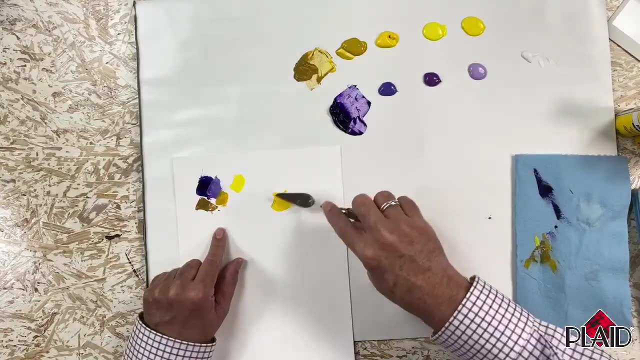 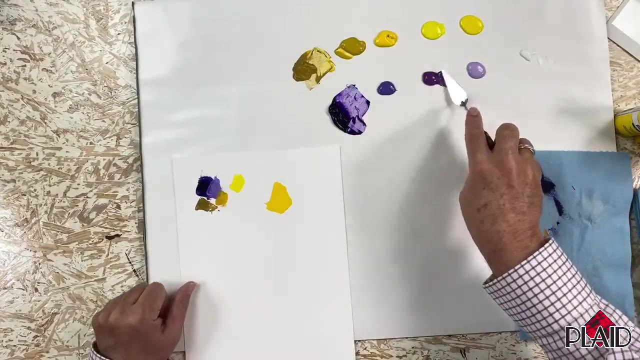 and bright contrasty lemons So you can make them the star of the show, however you want to do that. But let's take another yellow here and we'll just put a big swatch of this out here and we'll support this with a nice, more red-violet tone. 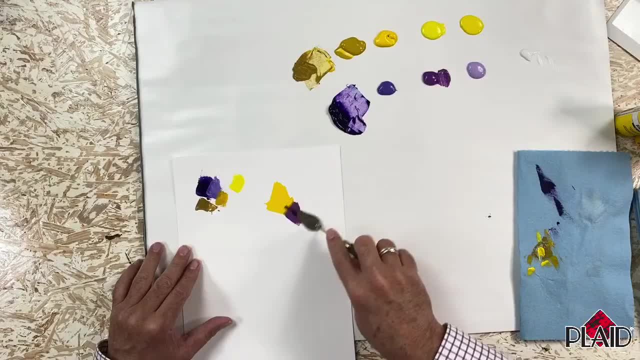 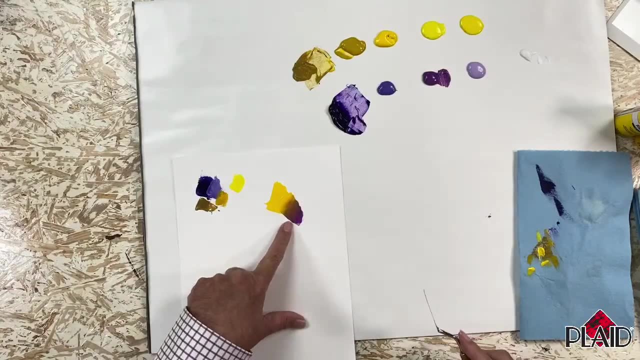 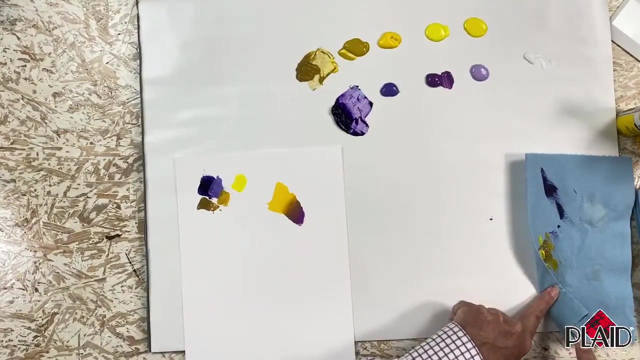 And those two sit pretty well together. We'll just mix and merge those so you could see how, by adding some of that yellow into that purple, you could get a whole range of colors here that will work well together in a painting and still allow your yellow to be the star, And, if we wanted to, even bump. 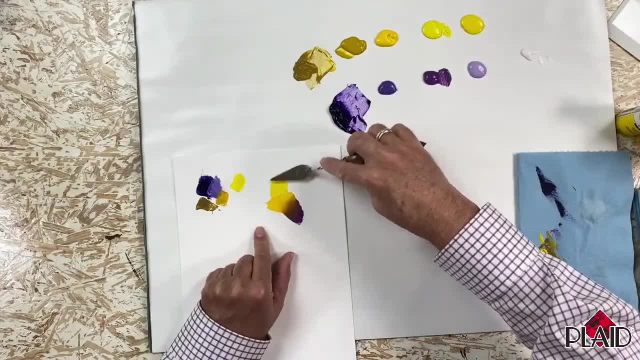 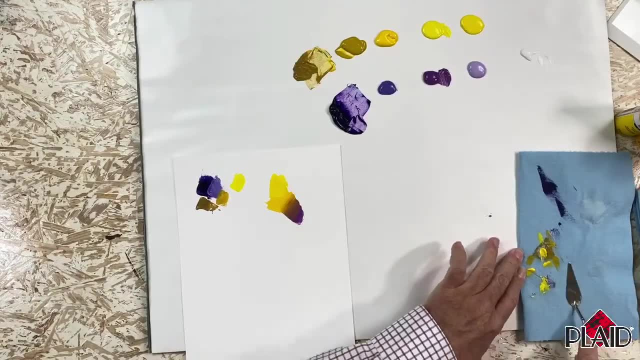 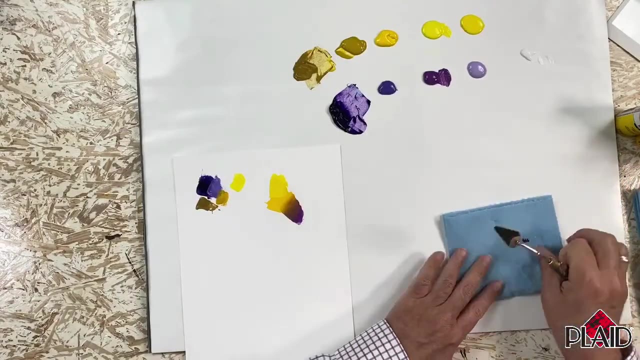 that contrast up a little more. we simply add some brighter yellow there and then the really does take your eye print. do we have any questions? so far, stephen? um, i think we are good. everybody's saying hello. but yeah, let us know where you guys are watching from and if you have. 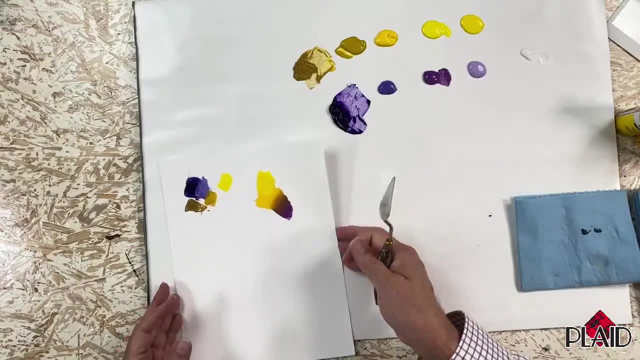 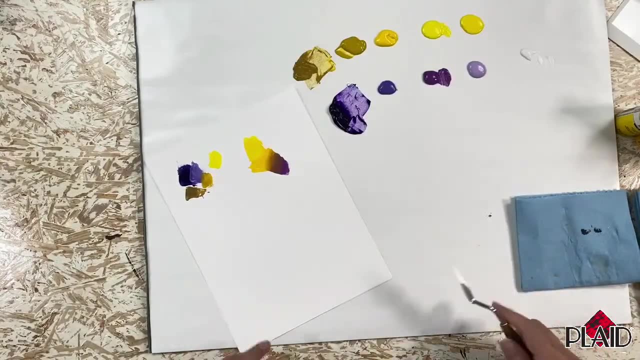 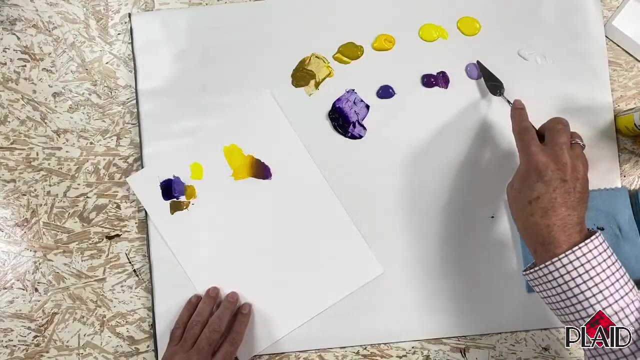 any questions for andy. okay, because this, this kind of stuff is. it's easy to, it's easy to play around in a paper, but when you actually start to put it into a painting it takes a little bit more effort. you have to mix little brains with your paint as you're working along. now let's take our a lighter. 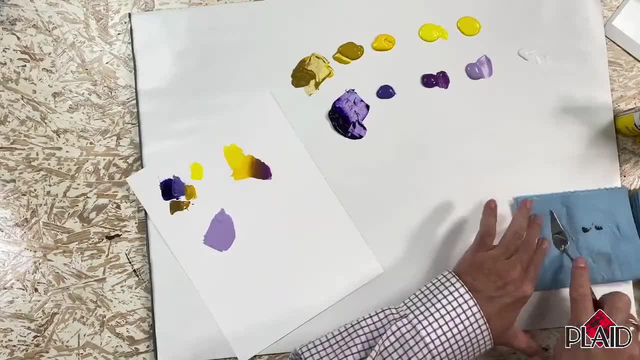 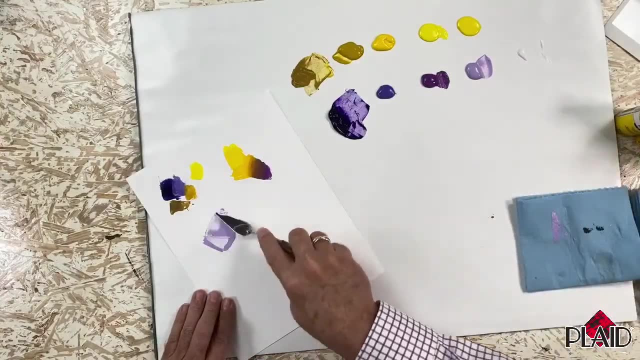 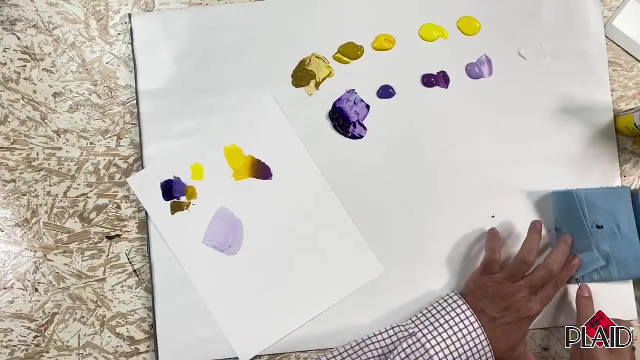 color purple here. so that's a light value purple, and we could go ahead and take a little of our titanium white and we'll just lighten this up right here on our paper. so we've got a very pale purple and we can pair that with a yellow. 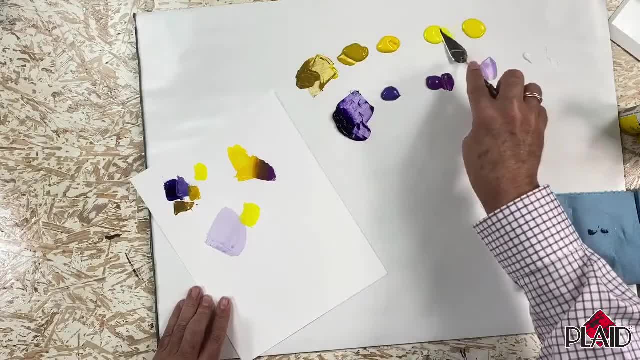 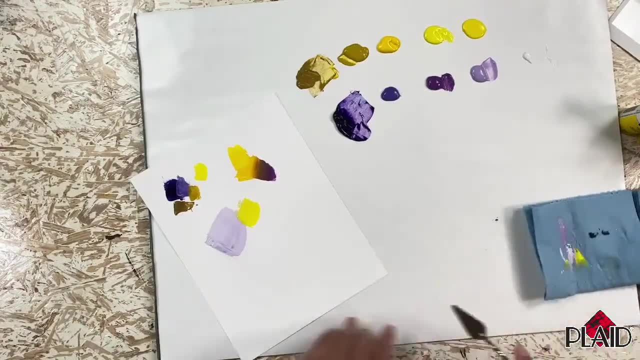 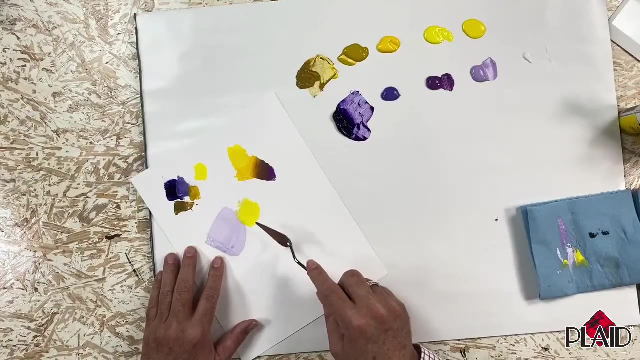 and this is very eastery to me and it evokes easter colors there- with the yellow and the purple. this very, very light lavender works very well with the light yellow and the yellow still is because it's such a intense color and we have made a tint of our violet, if you remember, back from. 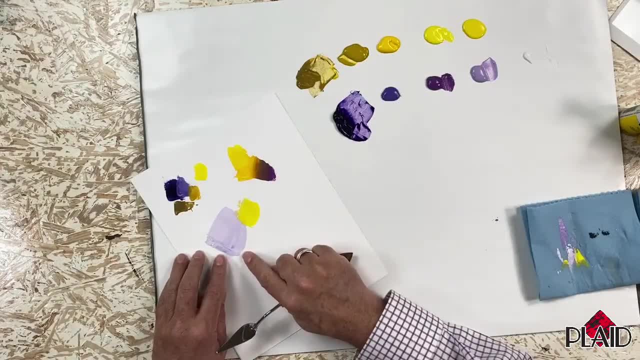 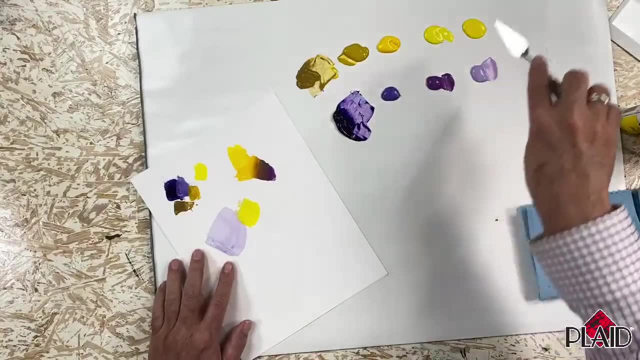 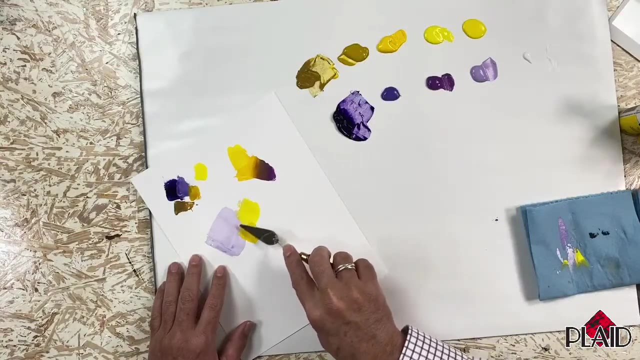 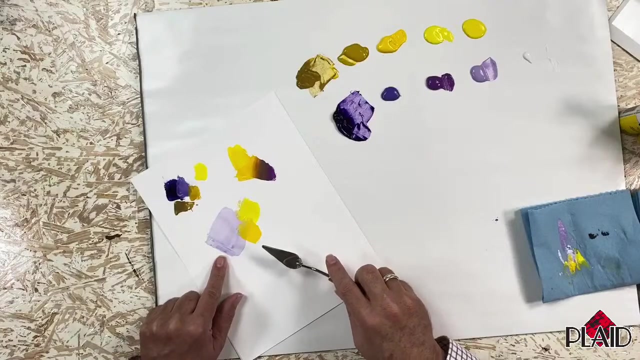 tense tones and shades. we added white here, so we have a tint of purple and a full intensity yellow there. so let's do a little bit deeper shade of yellow here so that you can see it works nicely there as well, and with this pale tint the yellow is always going to be the star of that show. 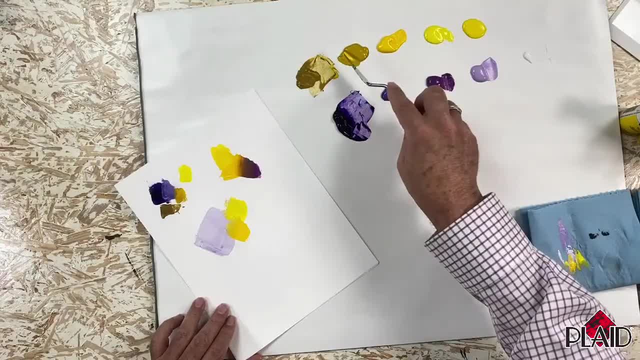 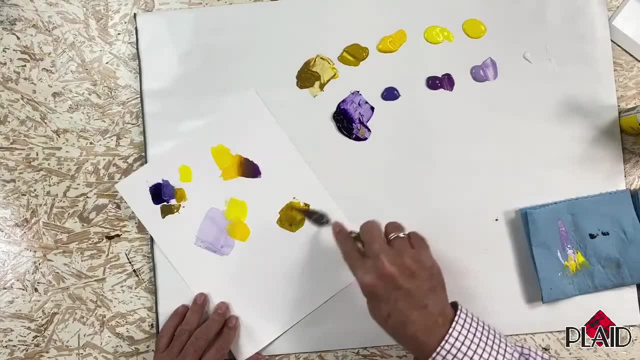 in order to make our purple the star of the show, we would have to start with a toned down purple. so i'm going to tone that with a little bit of a complementary color. we're going to tone it a little bit more. so far we're just working with the yellow and the purple, giving you 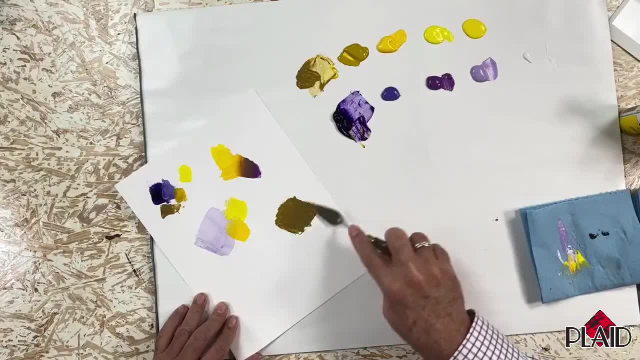 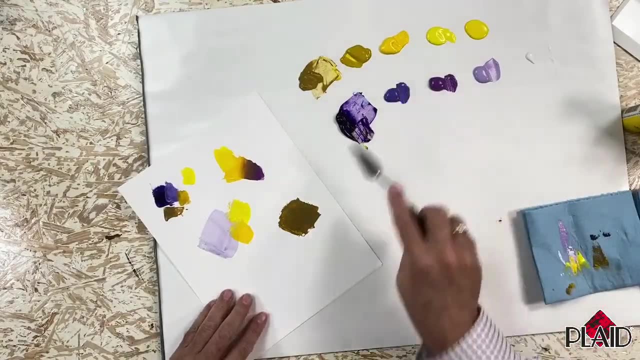 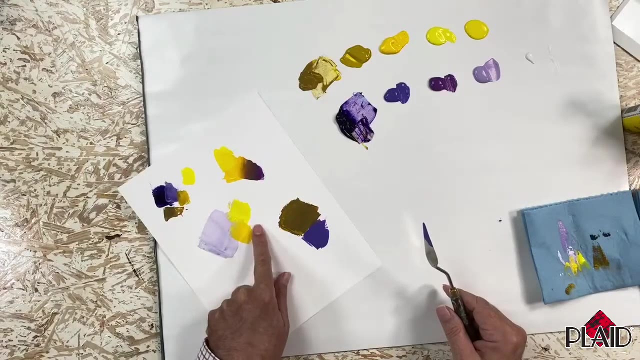 some information on how these colors look, but there's a very toned down yellow and i can take a bright purple and put that next to it and now the purple is the star of this show. here the yellows are the star, here the purple is the star, so it's usually going to be the color. 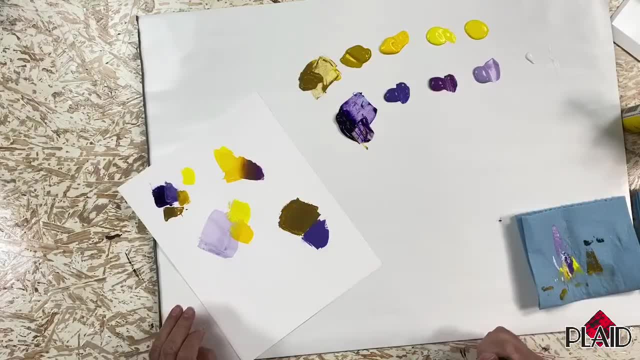 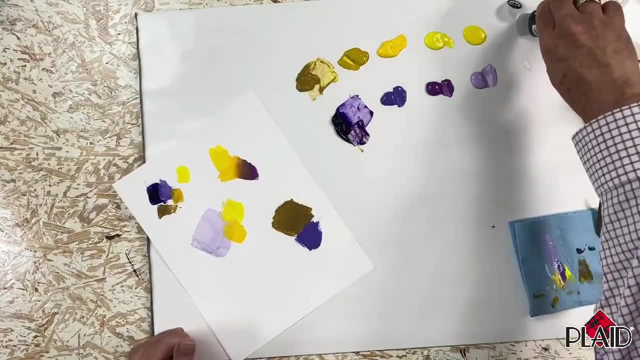 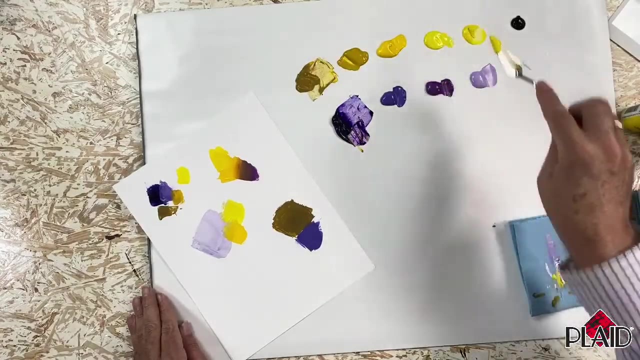 that has the highest chroma or the highest intensity. that's going to be the star of the show. but let's not forget that we can make a shade of a color with black. so let's take a nice yellow color here and let's make a shade of. 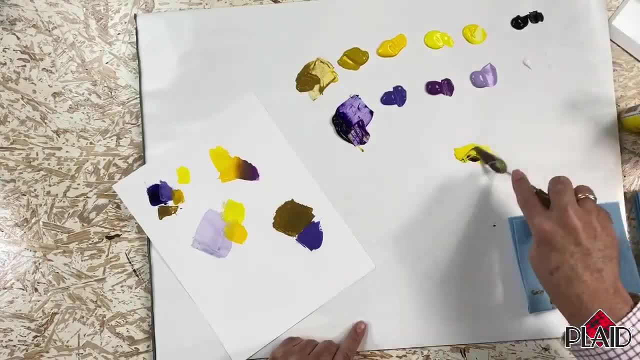 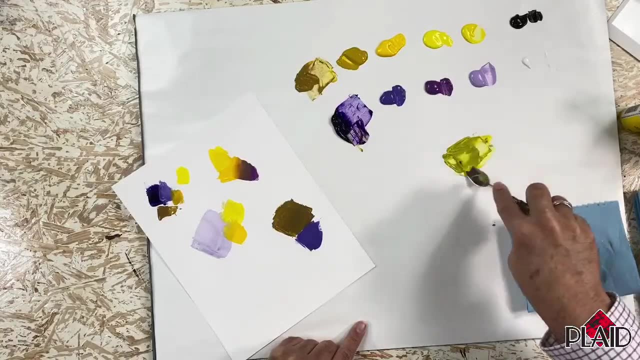 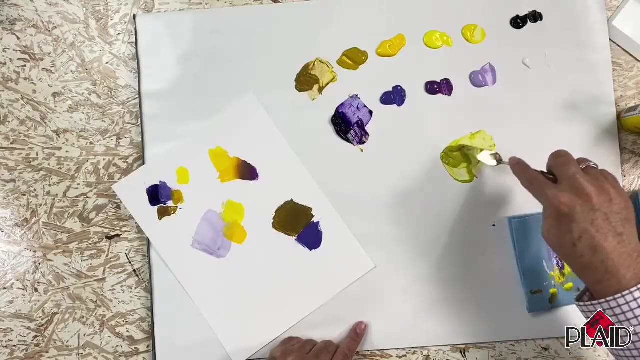 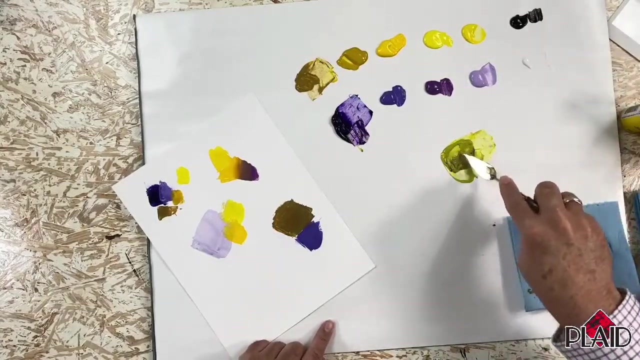 yellow with some black and hopefully, if i remember what my paints usually do for me, this is giving me a very nice green color. so let's just let's make a little darker tone or shade- actually sorry, this is a shade- it's hard to keep all those. 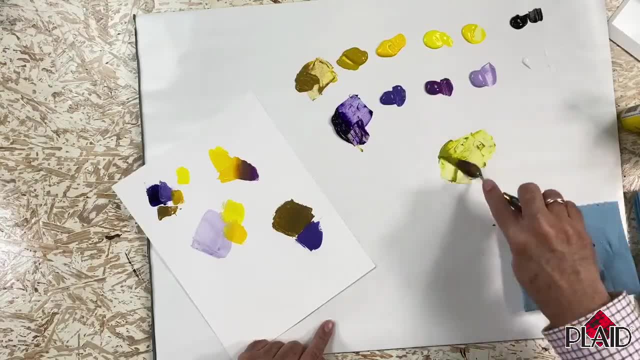 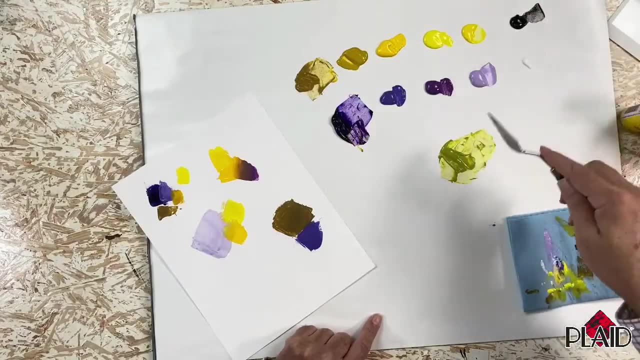 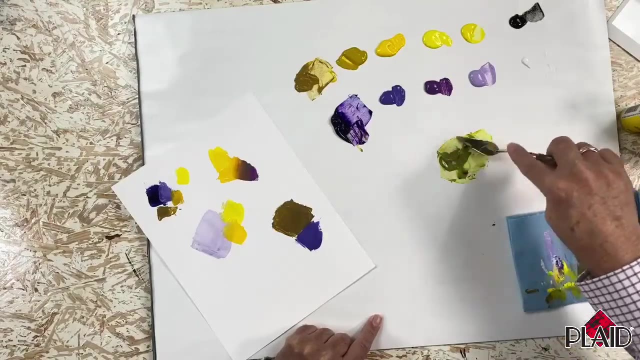 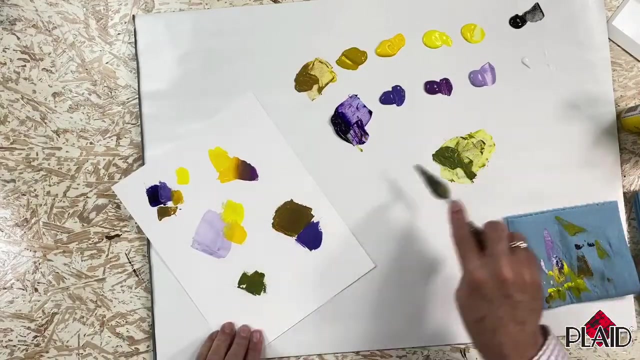 vocabulary words straight, all right. so we've made a shade of yellow here, and because i'm using black with yellow, i'm going to get a color that looks green. so if i needed to broaden out my color scheme a little bit, it's very easy to do, because now i've got greens, which of course could be leaves or whatever else. you might need in your design a little bit to get the color that you need. it's a lot easier to do because now i've got greens, which of course could be leaves or whatever else you might need in your design- leaves or something else you might need in your design. 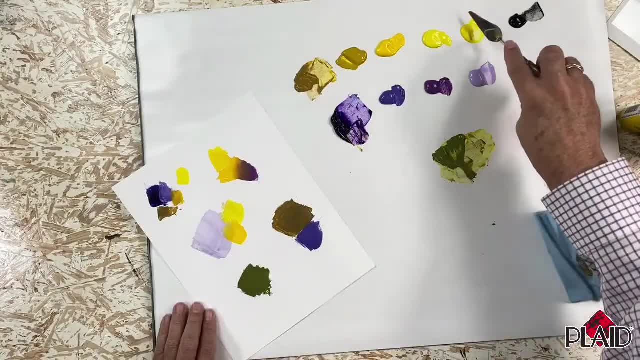 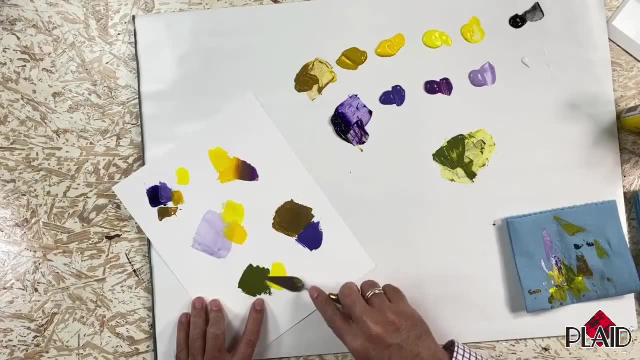 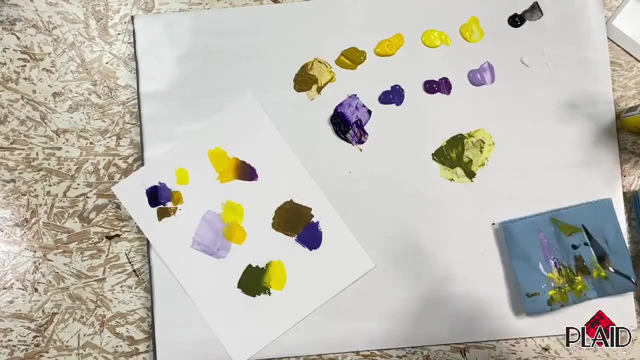 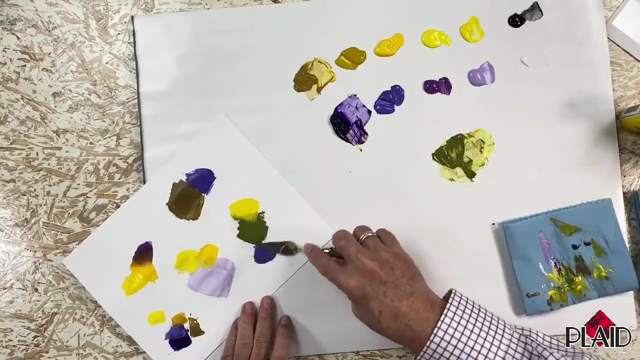 design. but we can contrast that shade of green or that shade of yellow with a high chroma, high intensity yellow. so your yellow is the star of that show. or if you wanted to show off a purple over here, the purple is now the star of the show with that shade of yellow there. 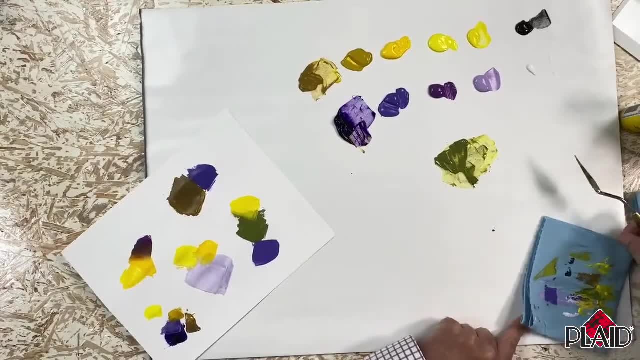 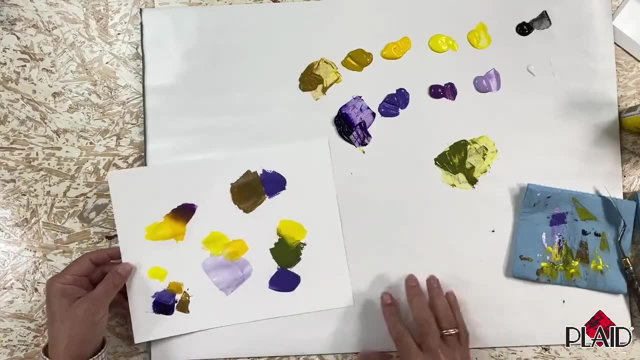 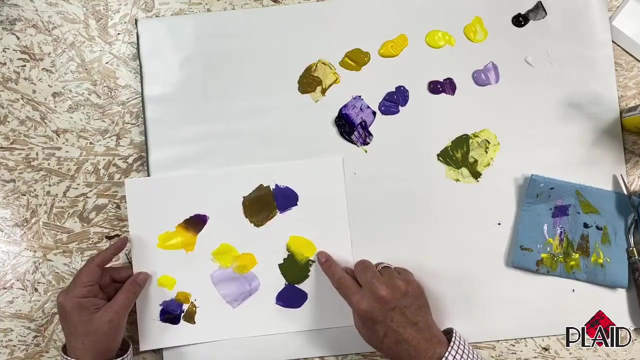 so don't let something like a complementary color scheme feel like you don't have options or choices, that everything needs to be fighting for attention. always remember that one thing has to be the star of the show, and here it could be yellow or it could be purple, because we are 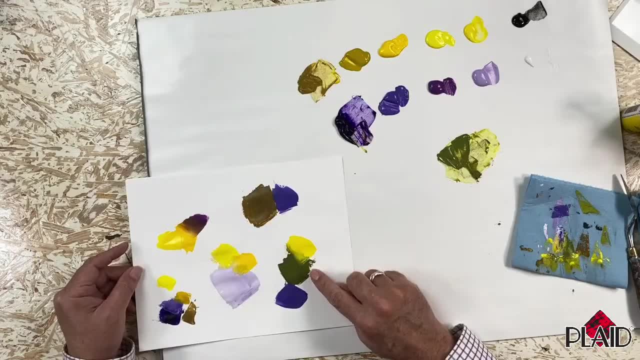 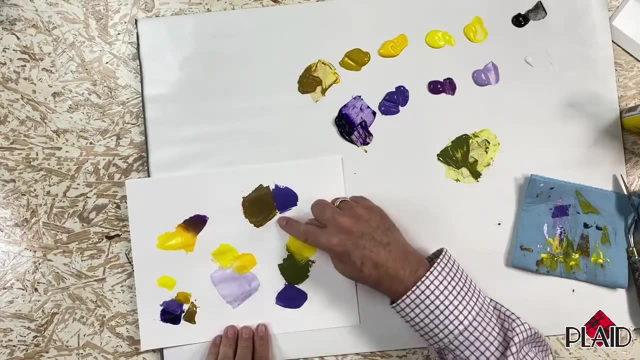 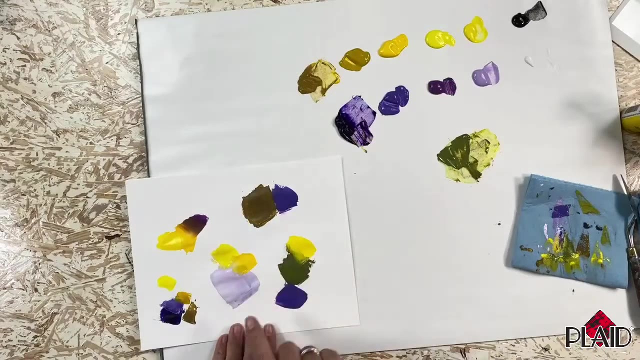 using that with a shade of yellow. here we've got our tint of purple and the yellow is completely the star. when we've done a tone of our yellow, we've let our purple be the star. so all of these color schemes are basically yellow and purple, complementary color schemes, but using these different colors. 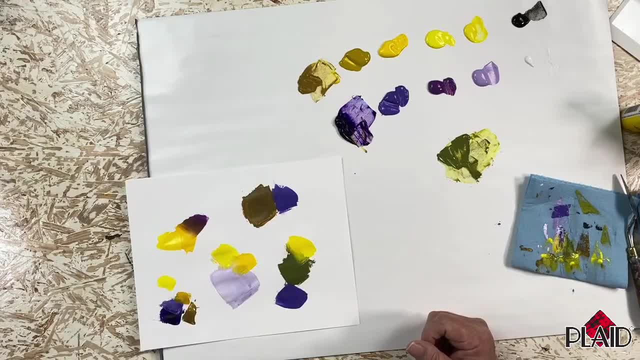 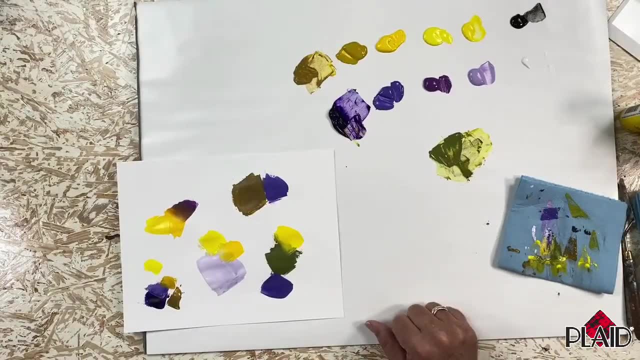 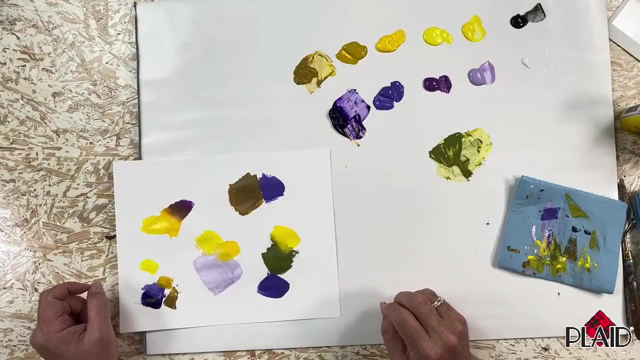 like this will give you wildly different paintings. so i'm going to ask again, steven, do we have any questions? anybody doesn't understand something. no, i think everybody is is understanding. okay. well, that's very good. this is just a the the the, the tip of the iceberg when it comes to complementary color schemes. so it would be great if somebody